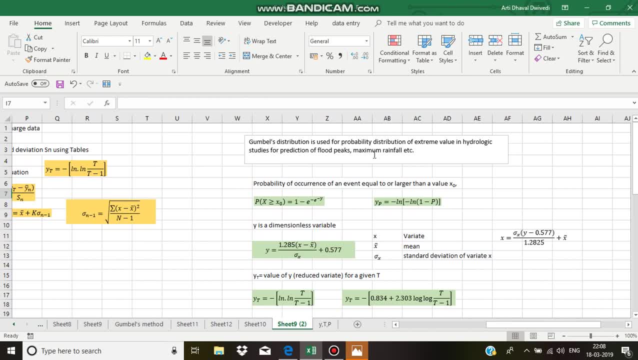 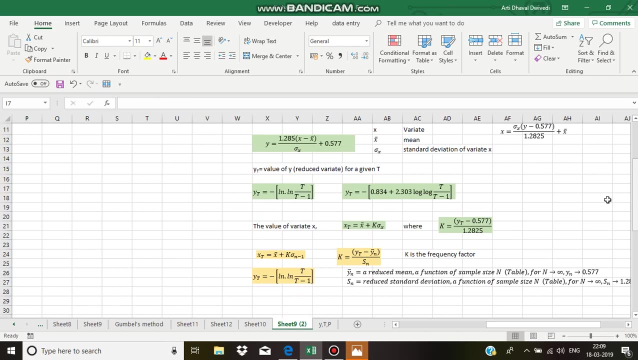 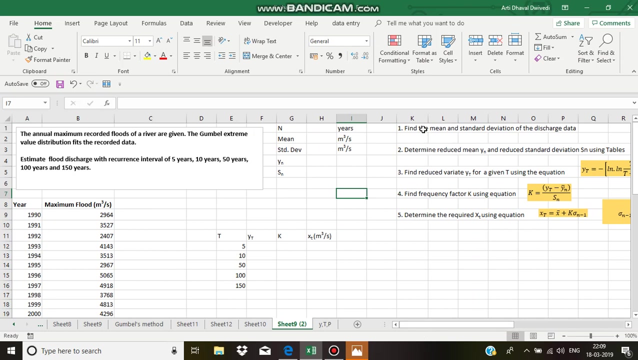 Now Gumbel's distribution is widely used for probability distribution of extreme value in hydrologic studies, for prediction of flood peaks, maximum rainfall, etc. And these are the equations associated with the Gumbel distribution. We will follow this procedure step by step to obtain the required xt, which is the maximum flood corresponding to the maximum flood. 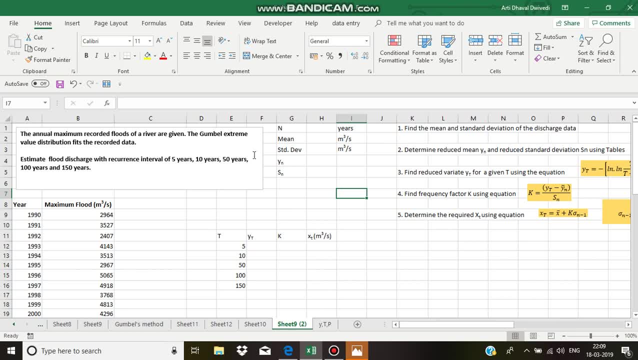 The number of flood barriers is divided into 5,10,50,100 years and 150 years. Let us find the mean and standard deviation of the discharge data. First of all, N is 27 years, 1990 to 2016.. 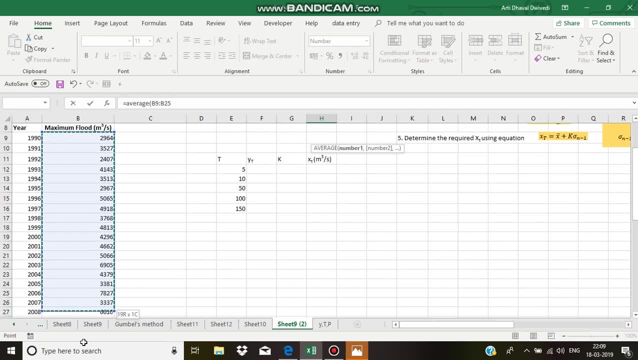 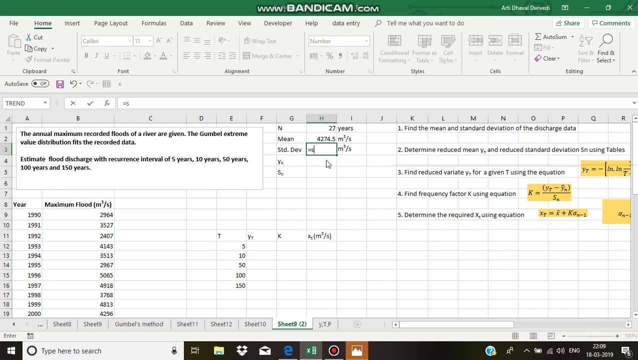 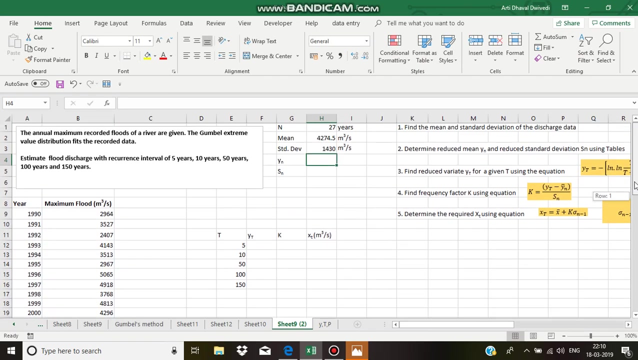 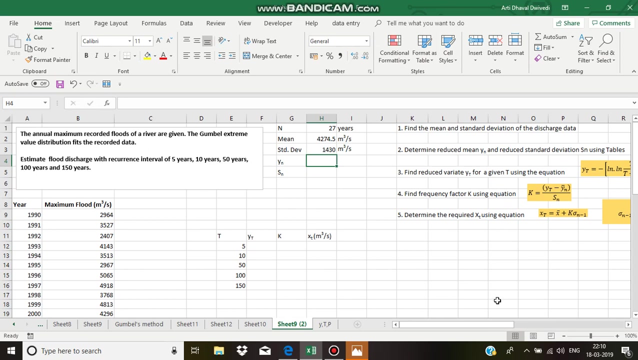 Mean average of these values is zero. standard deviation can be easily obtained using this stdv dot s. So the mean and standard deviation have been obtained. Now determine the reduced mean Yn and reduced standard deviation Sn using tables. So we will find out Yn and Sn which will be required in this equation. 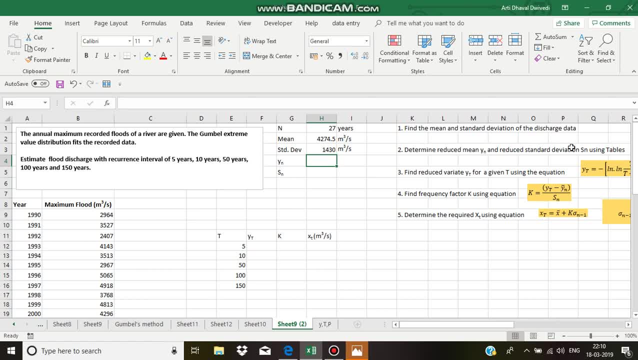 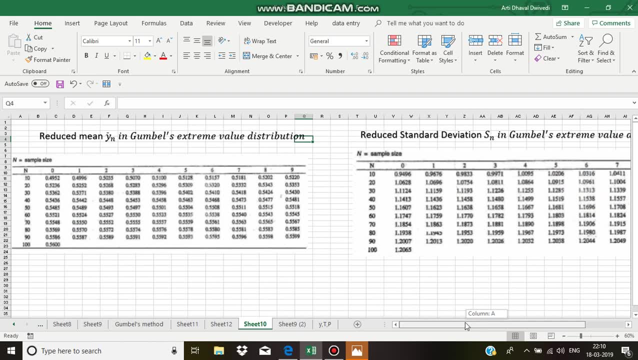 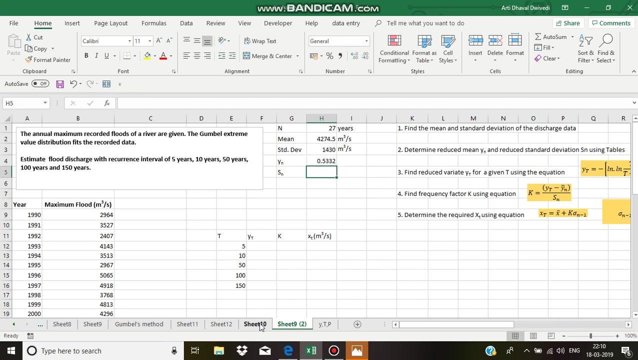 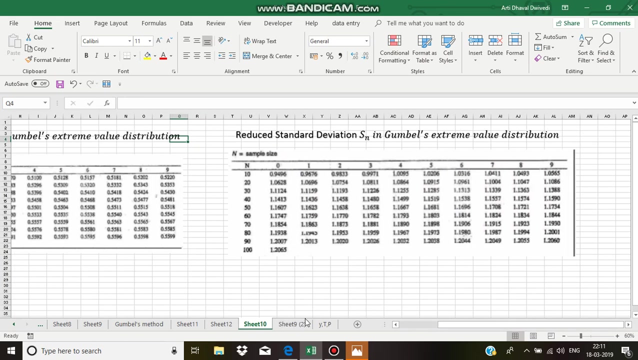 to find the frequency factor. So they can be found out from the tables. Now, the value of Yn, corresponding to the given sample size of 27 is 0.5332.. And value of reduced standard deviation, corresponding to sample size of 27, is 1.1004,, 1.1004, ok. 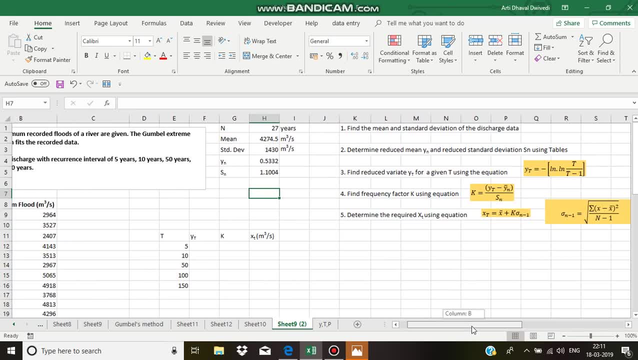 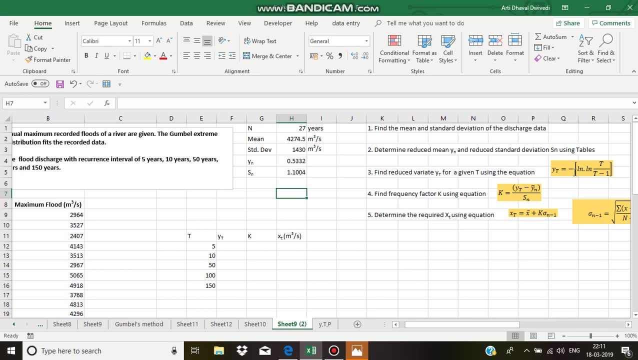 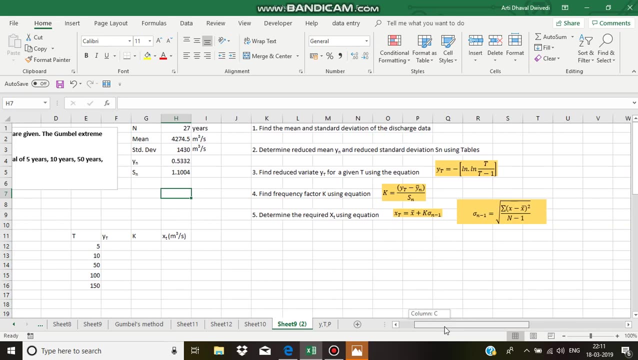 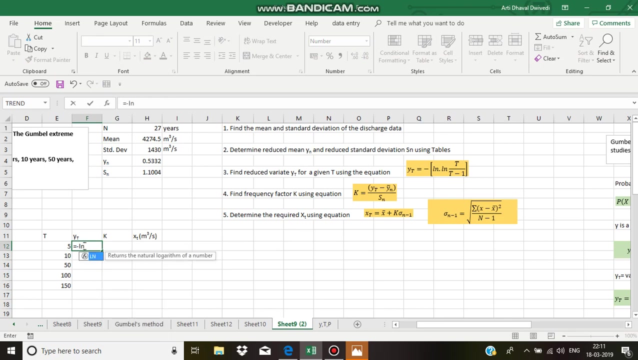 Now find the reduced variate for a given recurrence interval. using this equation, Yt is equal to minus ln ln t by t minus 1.. So Yt is equal to minus ln. natural logarithm, ln bracket, t square. So this is equal to minus ln ln t by t minus 1.. Now find the reduced. 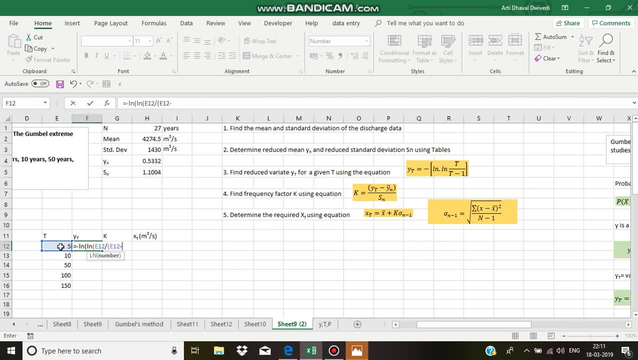 variable t by 5, divided by 5 minus 1.. The value of Yt reduced variate has been obtained. Now find frequency factor K. using this equation, K is equal to Yt minus Yn Ok 1. 5.. 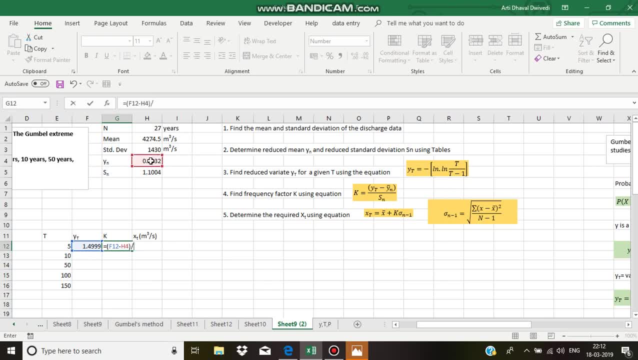 3., 7., 8., 5., 5., 4., 5., 6., 7., 5. divided by Sn. I will anchor these values so that they do not change. The value of frequency factor K has been obtained Now the value of Xt- maximum flood corresponding to recurrence. 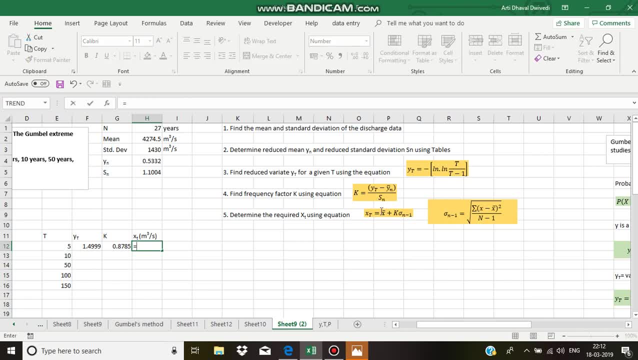 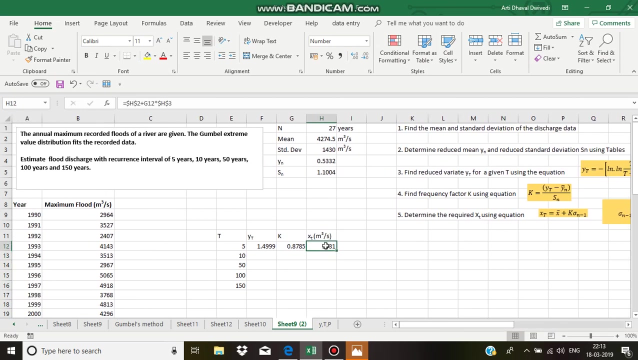 interval of 5 years can be obtained using this equation: Xt is equal to X bar, which is the mean. I will anchor this cell plus K, frequency factor K multiplied by standard deviation. So the value of maximum flood has been obtained. It is 5531 m3 per second. Similarly we can 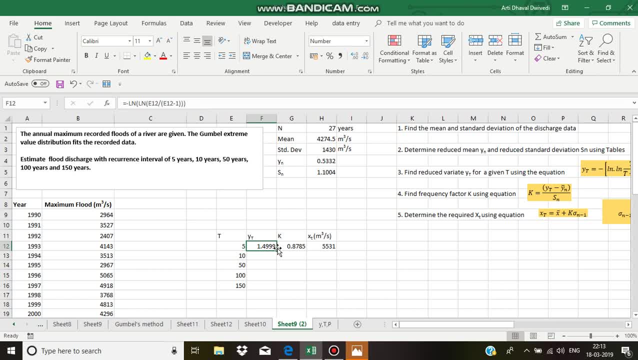 find out Yt for 10 years, 50 years, 100 years and 150 years. corresponding frequency factor K can be found out using this equation. and then the value of Xt can be found out using this equation. This is the maximum discharge corresponding to recurrence interval of 150 years. it is: 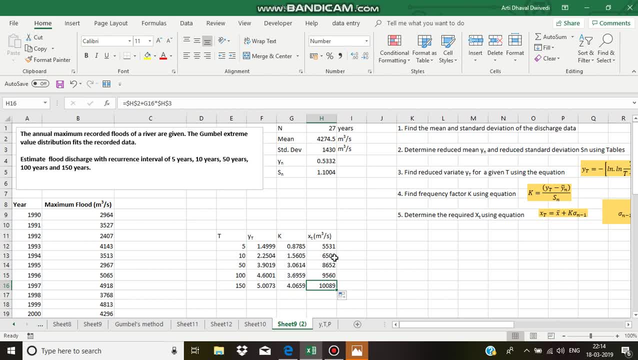 10089 m3 per second. It is 6506 m3 per second for recurrence interval of 10 years, 8652 for 50 years, 9560 for recurrence interval of 100 years. Now these values can be plotted on Gumbel's probability paper and Gumbel's probability. 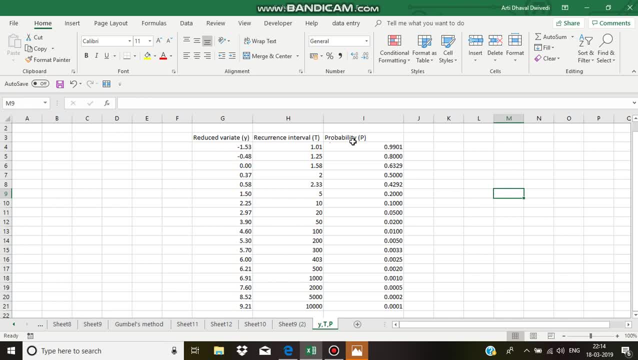 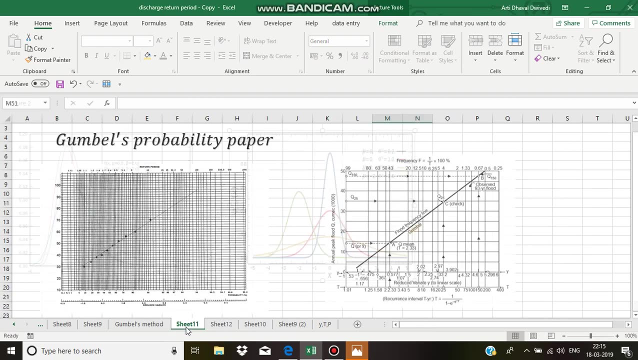 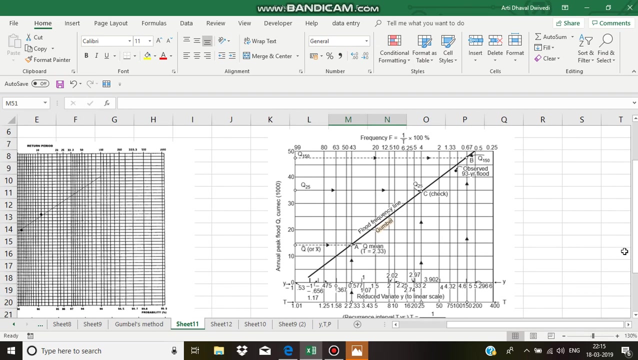 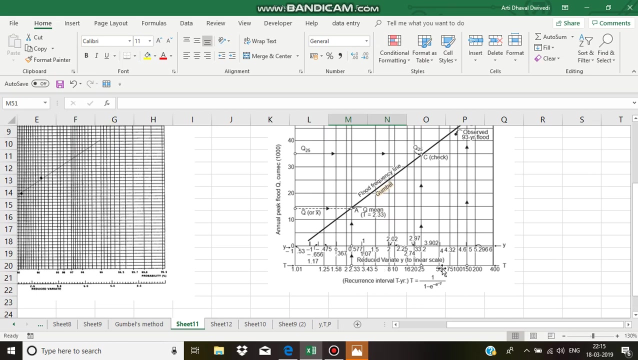 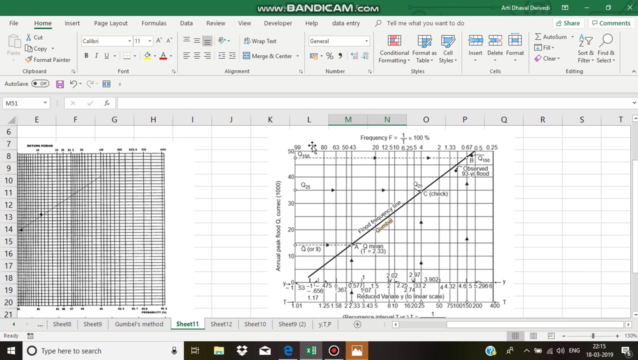 paper uses these values on its x-axis- reduced variate, y, recurrence interval, t, probability- and this Gumbel's probability paper would look something like this: Here is the reduced variate, here is the corresponding recurrence interval, and on the x-axis there is frequency or probability equal to 1 by t. 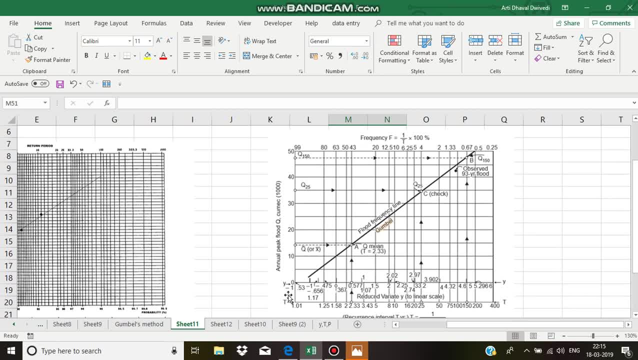 So we have the value of t, y and frequency or probability on the x-axis and value of annual peak flood. So this would be 1 by t. So we have the value of t, y and frequency or probability on the x-axis and value of.